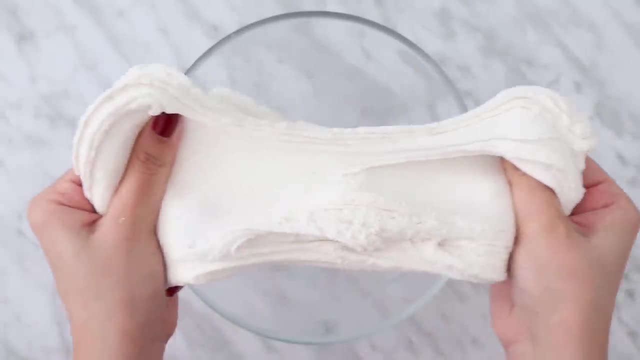 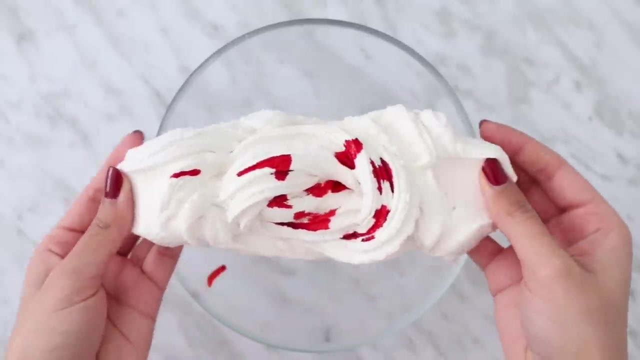 Even growing them out so that the slime will not be unfamiliar to the people around too much. the clay is stretchy, so I'm gonna go ahead and add a few drops of food coloring just to give it a nice color. so I added in like a lot of red to get a 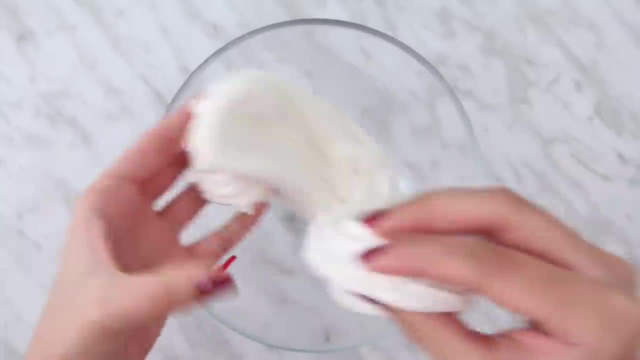 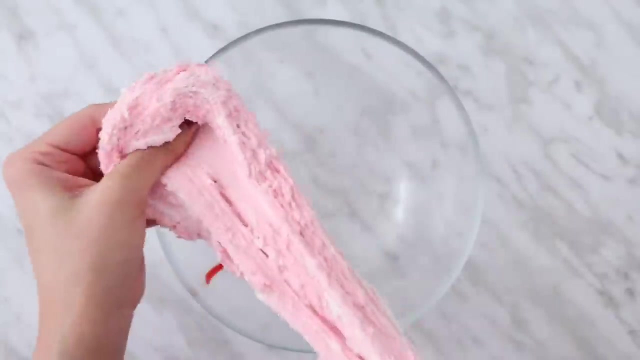 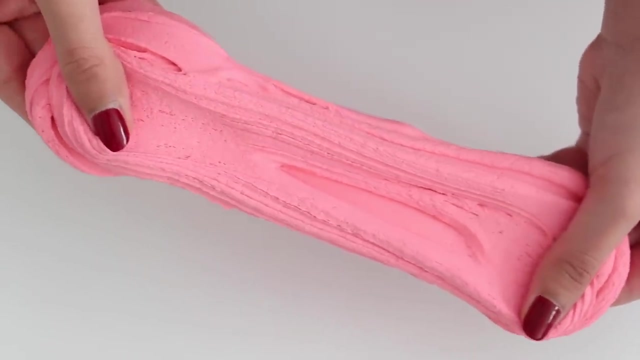 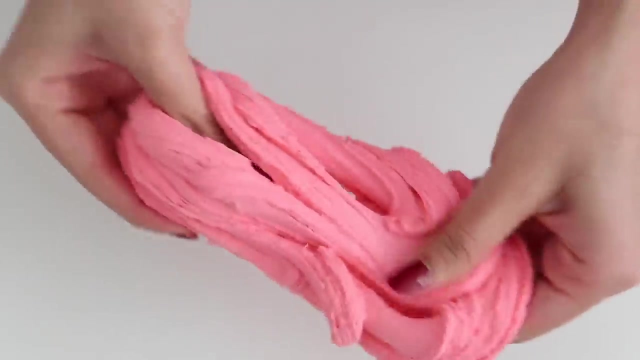 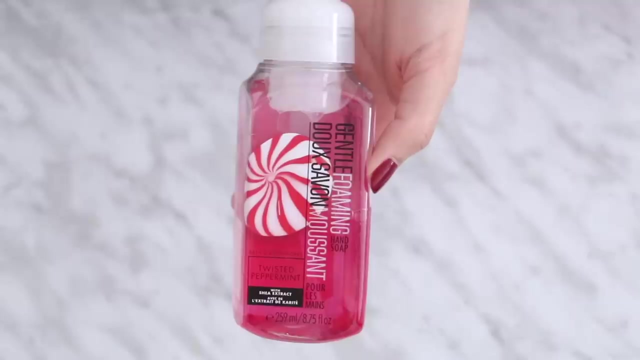 very nice and bright pink. this is, hands-down, my favorite no glue and no borax slime recipe. this has such an amazing texture to it. it kind of feels like butter slime. it's very stretchy and it also spreads very nicely. for the next slime recipe, you're going to need blue tack and some foaming hand. 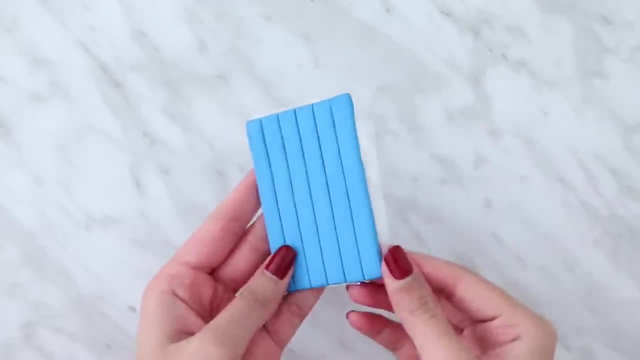 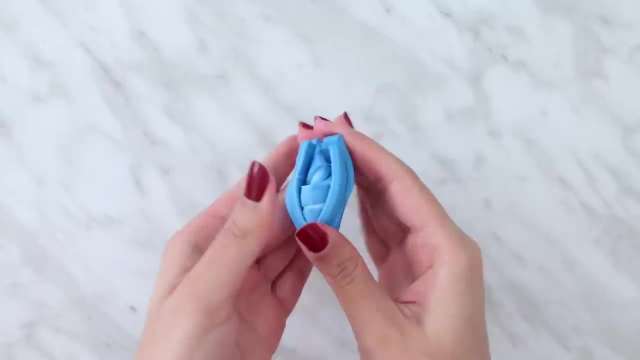 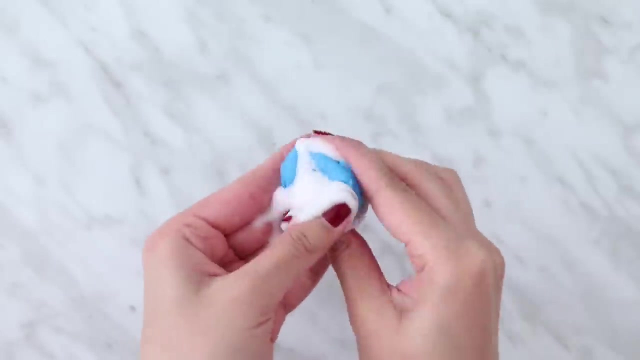 soap. so I'm gonna take the blue tack and just start working with it, using my hands, just to soften it up and to kind of get it a bit stretchy. I'm going to add in about three pumps of the foaming hand soap and I'm gonna 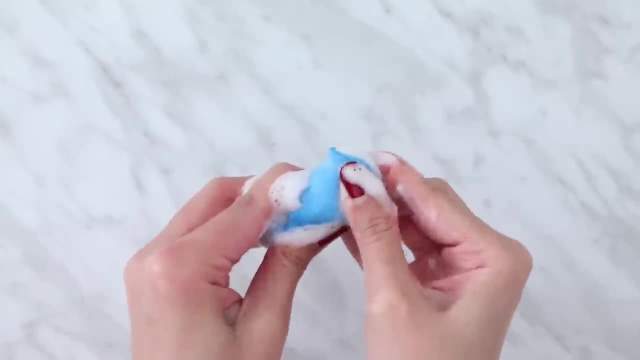 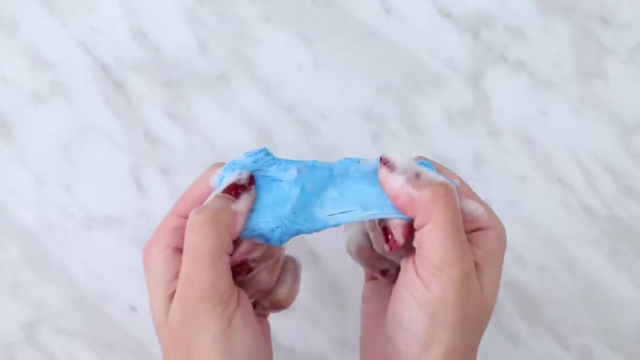 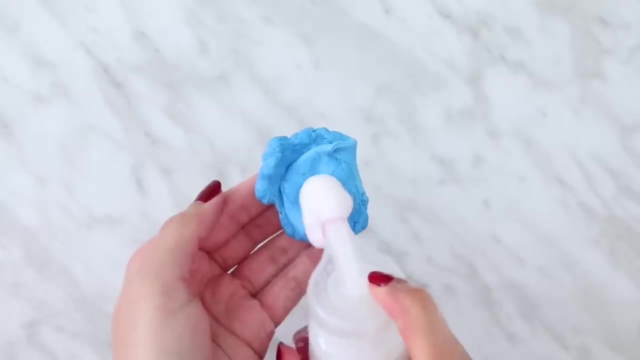 start working with it using my hands again. I'm doing the same thing like I was doing earlier. I'm kind of mushing it and trying to stretch it. now it will start kind of breaking apart, but you want to keep adding in foaming hand so and you do want to keep adding this in until it gets stretchy like actual slime. 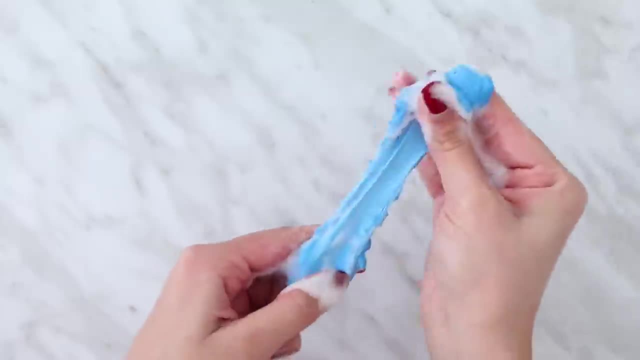 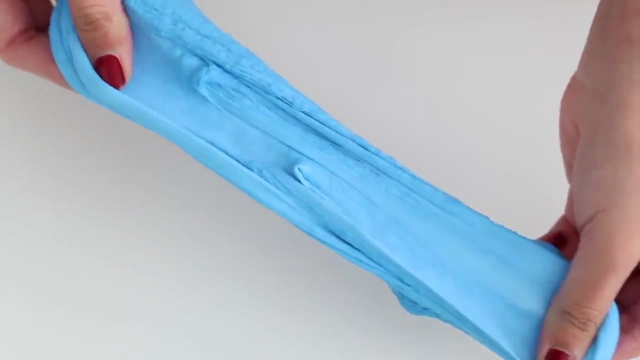 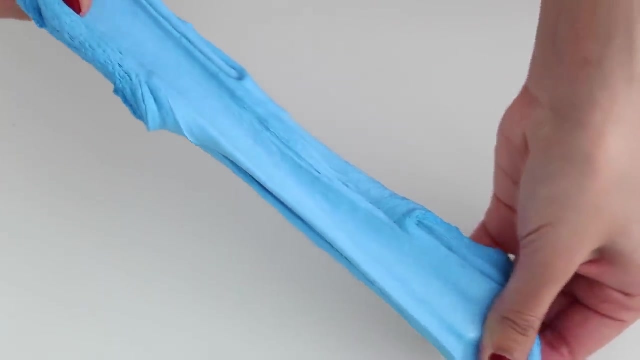 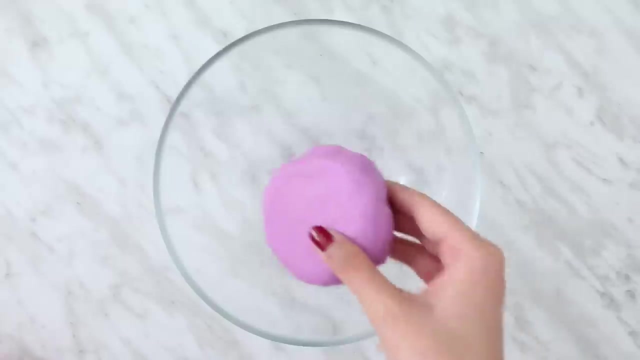 so this slime is very stretchy, as you can see. it's not as spreadable, but it is very stretchy, just like regular slime. for this next slime recipe, you're going to need play-doh and body lotion. I'm using the same body lotion that I was using earlier and it's pretty much the same. 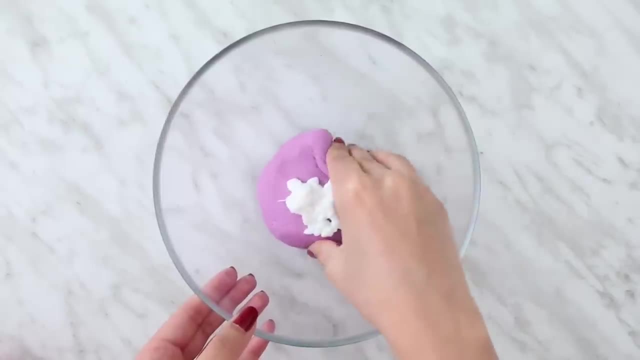 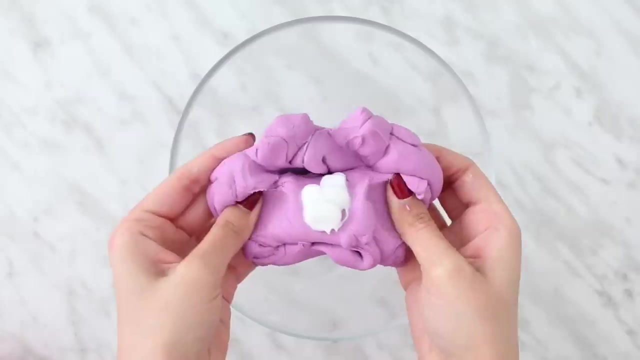 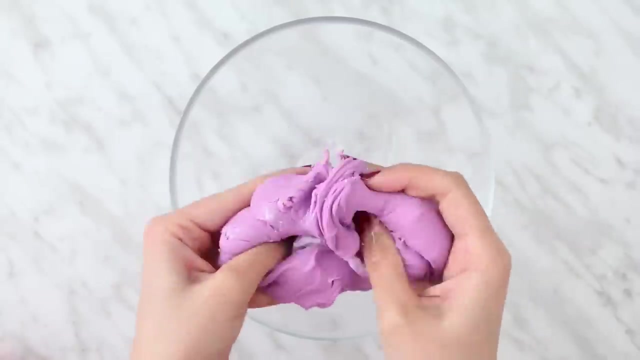 thing. you want to go ahead and add in a lot of body lotion and start kneading it into it. you want to keep adding in the body lotion until it gets very soft. so this one isn't as stretchy like the previous ones we made. so I'm just going to add in a little bit of body lotion and start kneading.